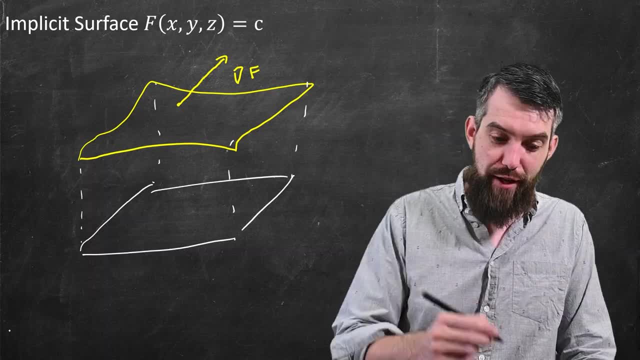 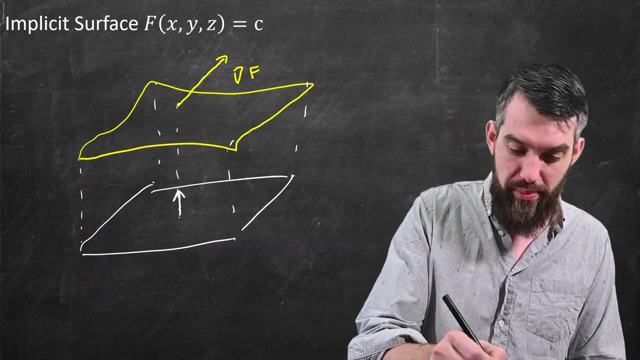 normal vector that will be normal to the surface at that point. If I go straight down into the x y plane, there's another vector here. There's a vector that actually points straight up. That's the normal to the x y plane, which is the vector k hat. So now, 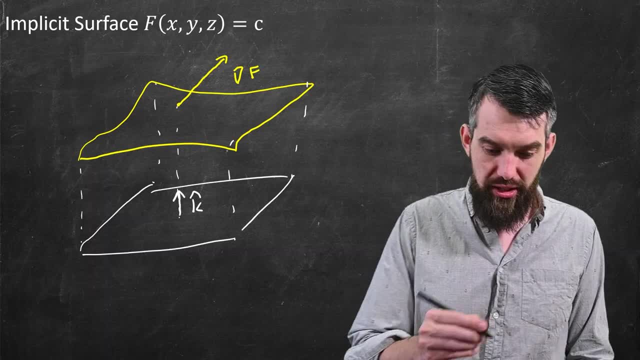 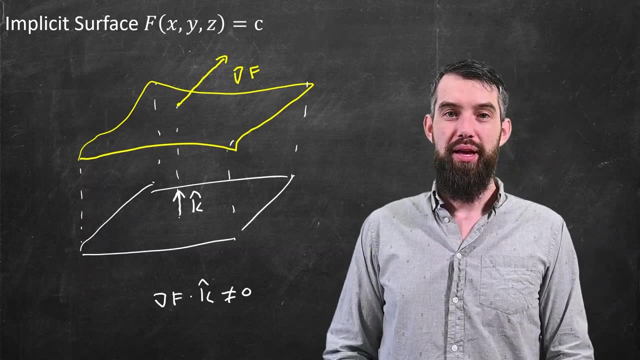 I get to tell you the type of surfaces I'm talking about. I'm talking about surfaces where that gradient vector and that k hat vector are non-zero, That is, there's no point where k hat is pointing straight up and the gradient, for example, is straight horizontally. 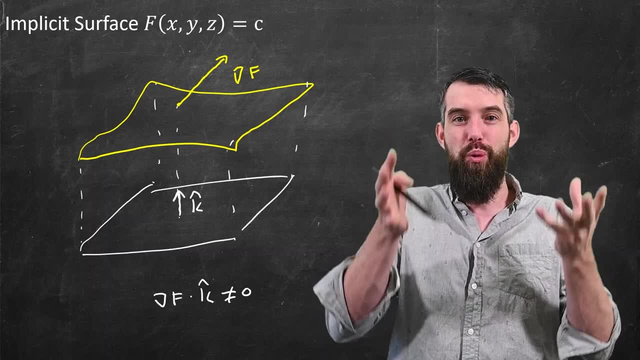 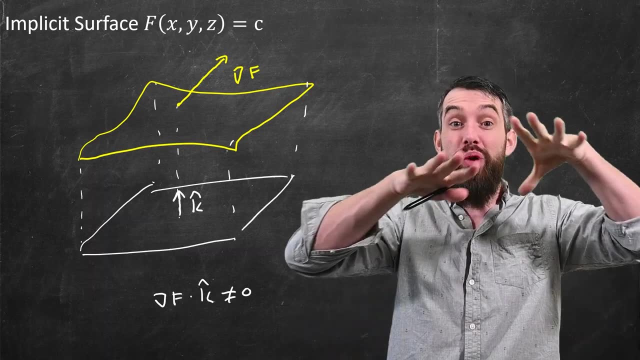 I'm talking about one where the gradient of f always has at least some upwards component to it, such that this dot product is non-zero. And that is the sense in which I'm going to talk about my region, of my surface being above the x y plane. We're going to see in a moment. 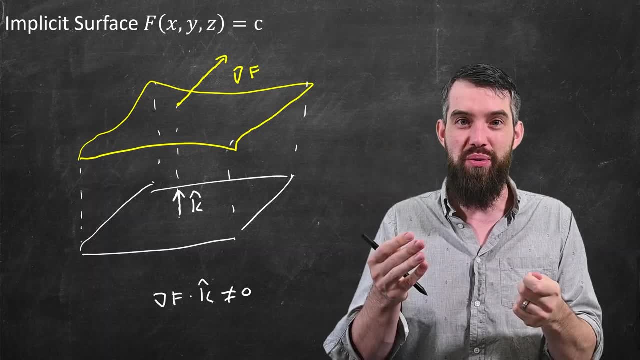 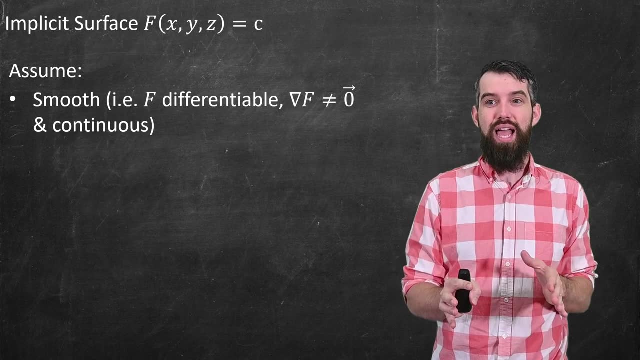 this is going to be very important in terms of not having a denominator of zero in the formulas we're going to compute. Now I'm going to talk about the assumptions a little bit more precisely. The first thing I'm going to assume is that I have a nice surface f. 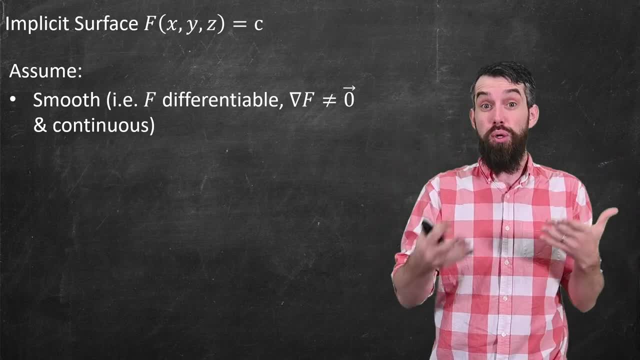 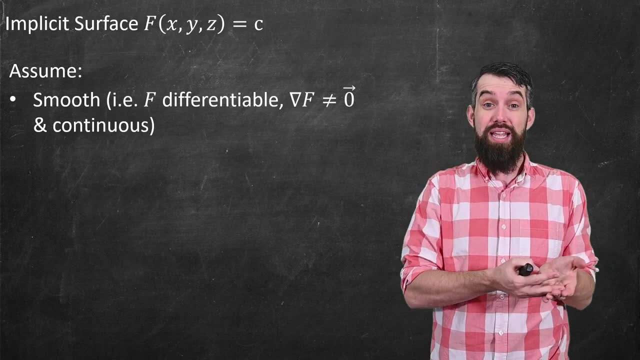 And what I mean by nice is specific, Specifically that it is what we call a smooth surface To form the gradient of f. you're taking the partial derivative with respect to each of the different components And what I'm saying is that those partial derivatives need to result in a gradient vector, which 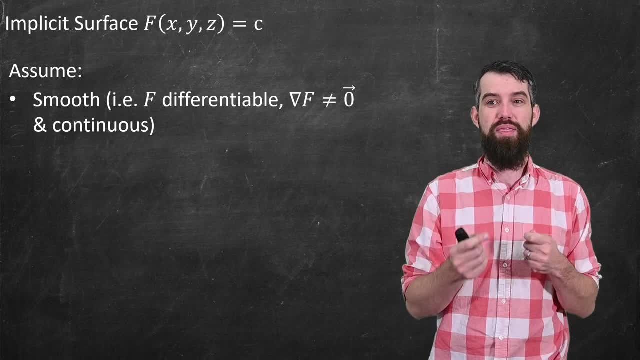 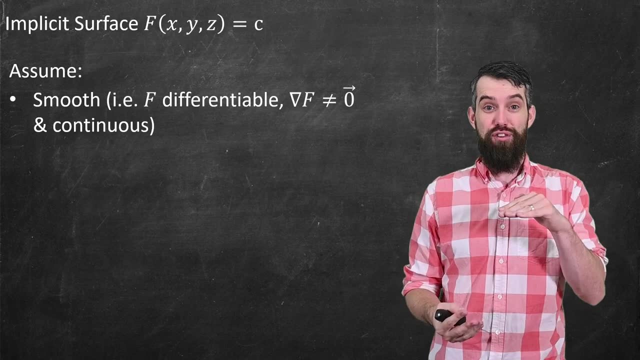 is continuous. But in addition I'm going to also demand that the gradient vector is not at any point the zero vector. But basically what I'm saying is that any patch of surface, there really is defined two unit normals, one sort of pointing up and one pointing down. 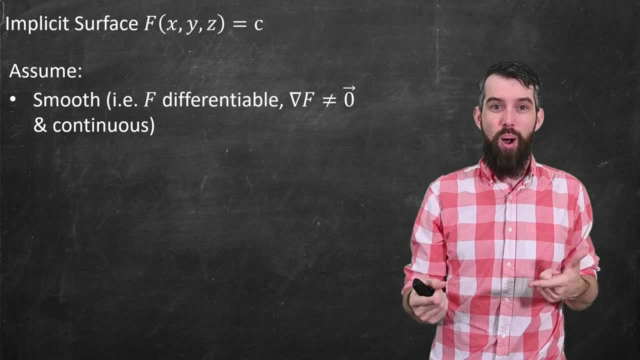 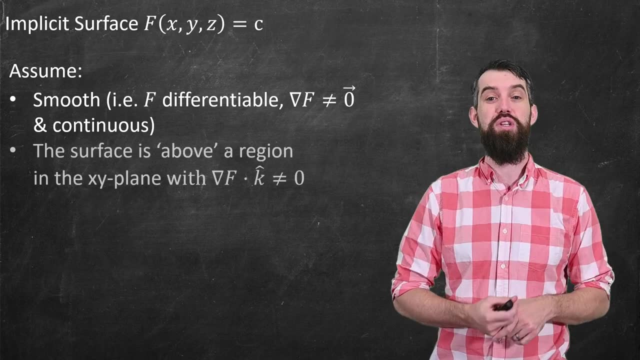 for any particular patch of surface that you have. There's no degenerate spots where the normal vector is just zero. So I need that for my surface to be relatively nice. And then, secondly- it was what we talked about previously- I want to think about this surface. 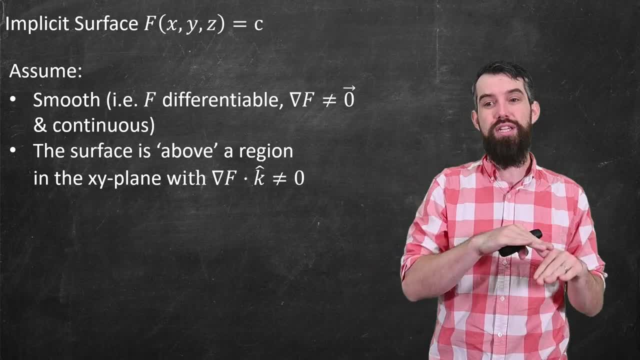 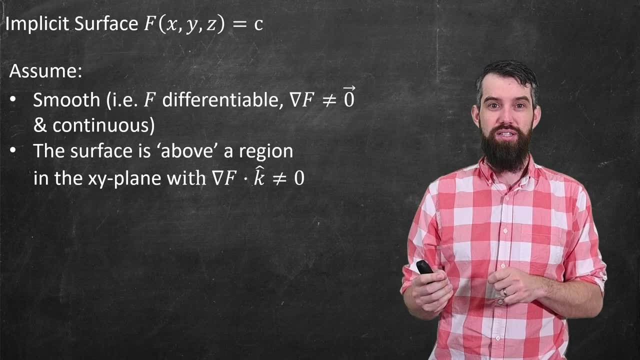 as being above a particular region down in the x y plane, And what I mean in that sense is that the gradient vector dotted with k hat is non-zero. So this is just to exclude the possibility that you have your x y plane down here And 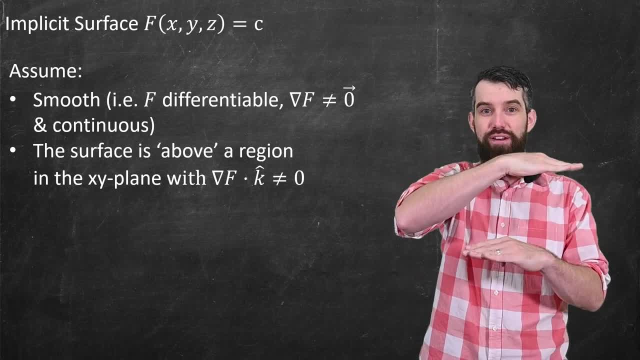 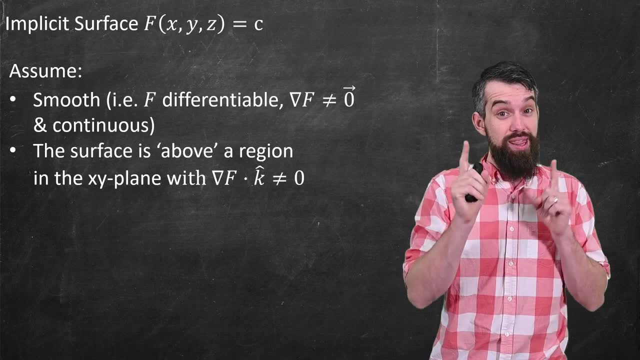 say, for example, you had a straight vertical surface where the gradient vector would be parallel to the original surface, would have this dot product of zero. Okay, so given those two assumptions, then we get our formula Here. it is The surface. 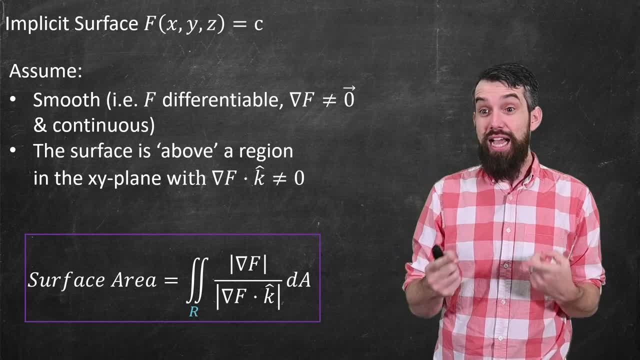 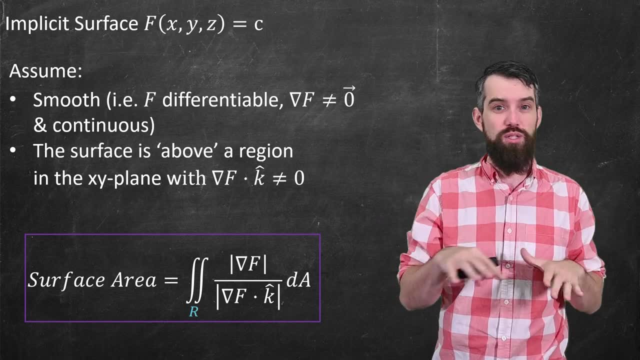 area is the double integral over a region in the x? y plane. So it's saying that I'm above a region in the x? y plane. You take an integral with respect to area in the x? y plane, so a, dx, dy, And then my integrand is the magnitude of the gradient of f divided. 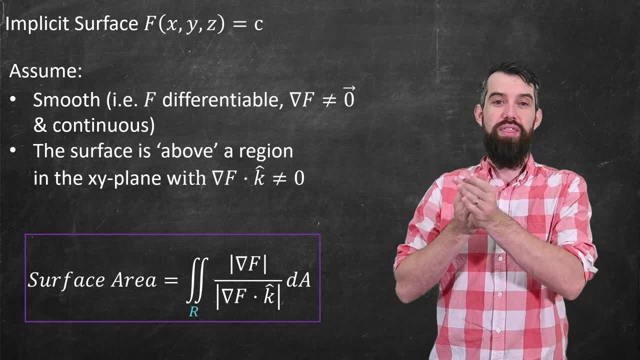 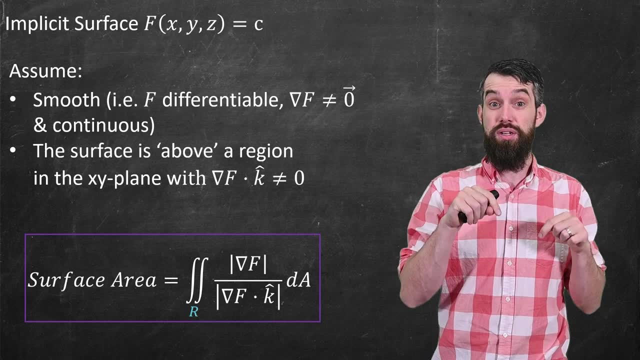 by the magnitude of the gradient of f dotted with k hat. And notice here in our formula how important it was that the gradient of f dotted with k hat was non-zero because that's down in the denominator. Now, when we proved the analogous surface area formula for parametrically described, 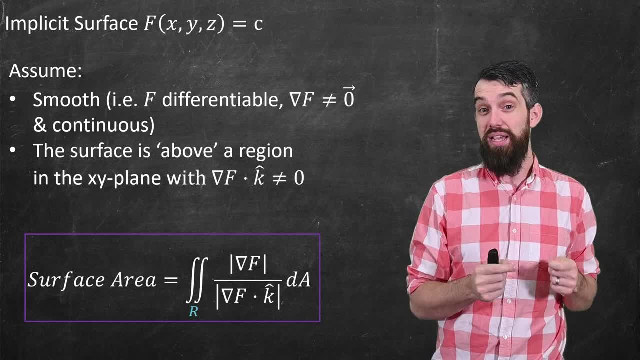 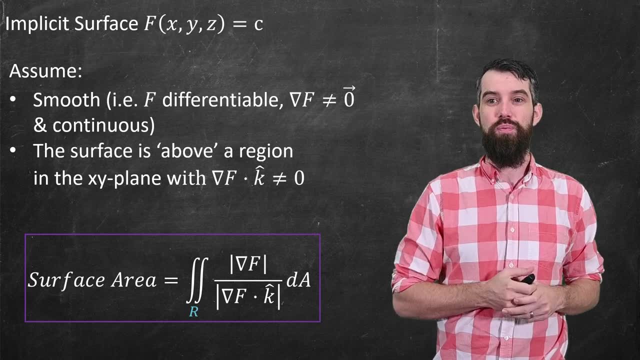 surfaces. I spent a bunch of time on the derivation. I'm not going to do the same thing in this video, That is, I'm going to skip the sort of formal derivation as to why the surface area formula is true, but I do want to motivate it just a little bit. So one thing. 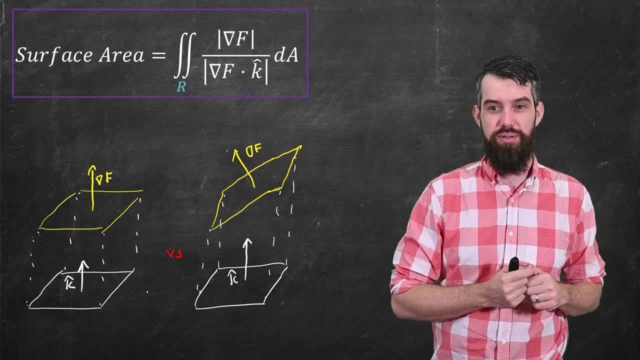 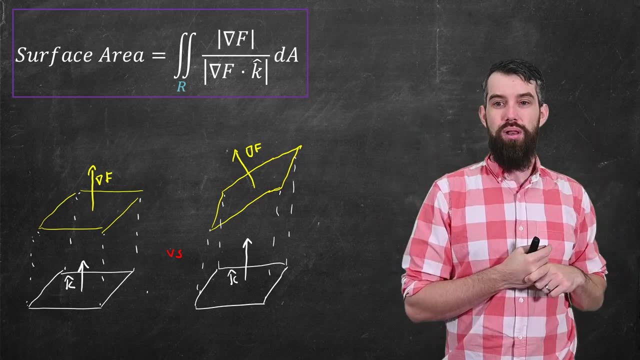 I want to focus in on is a contrast between two different scenarios. So in both scenarios I have a gradient of f that's got the x- y plane, And then I have a surface that's living above it. Well, on the far left, I'm imagining that my surface is completely flat, directly. 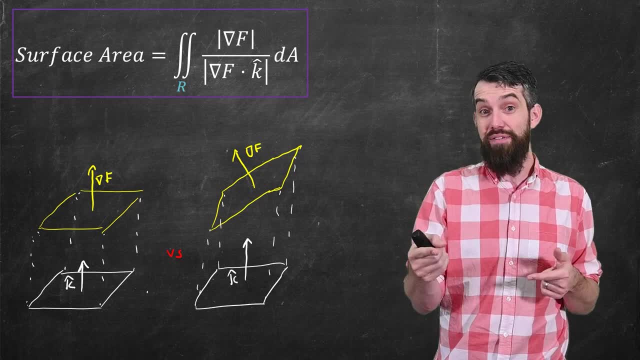 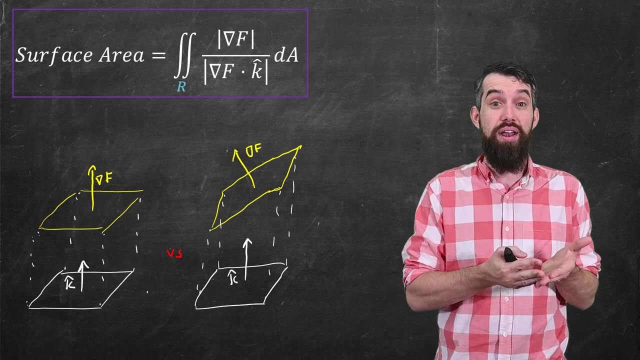 above the portion on the x- y plane. So in this case, the length of the gradient f and the portion of the gradient of f that's in the k hat direction, those are just the same And so this integrand is just one, and integrating out the area along the base is going to give. 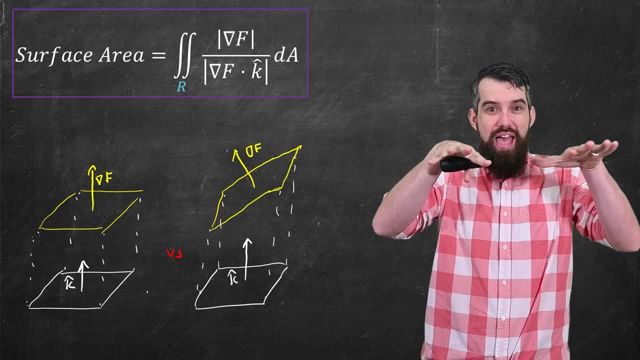 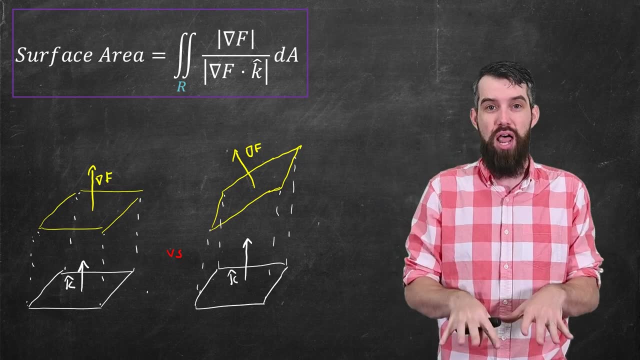 you the surface area, But in the second that surface is now twisted. It would take more material to paper over that tilted surface than it would the underlying one in the domain, And so what we need to have is a stretching factor And gradient. 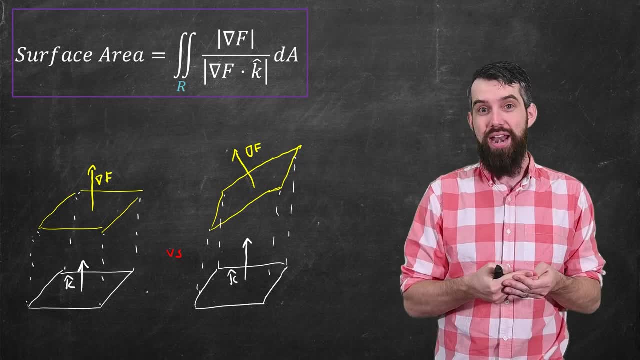 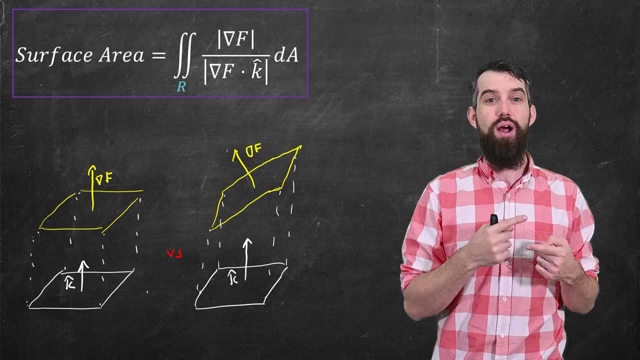 of f divided by the length of the gradient of f-dot and k-hat gives us that stretching factor. Indeed, the more the plane is twisted, the more the gradient of f-dot, k-hat gets smaller, And if it's smaller than the denominator, it's bigger. 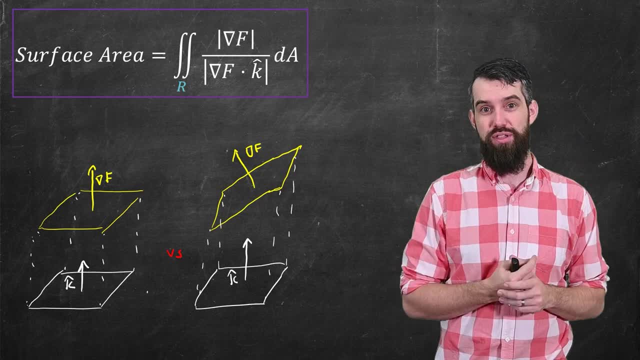 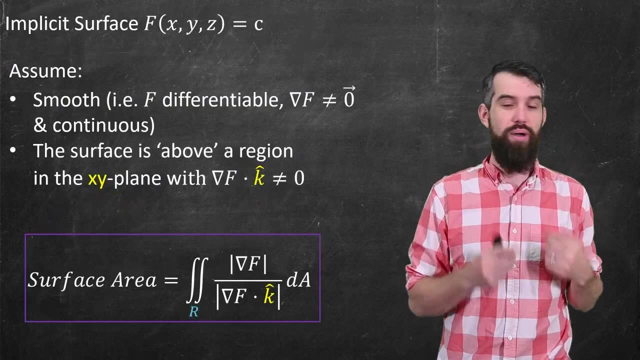 overall, Basically, we've got a ratio between the original length of the gradient vector and then this portion of the gradient vector in the k-hat direction. That is our scaling factor. Okay, so returning back to our statement with the assumptions, The actual assumption that it was over-origin in 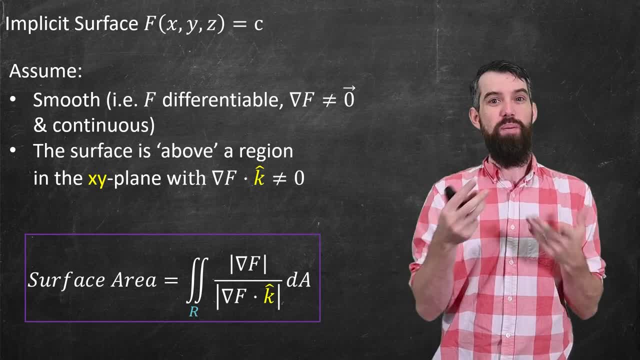 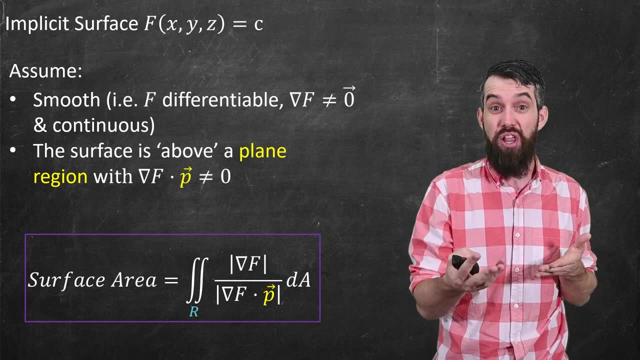 the xy plane and that we were dotting it with k-hat was actually a little bit arbitrary. In fact, I could replace this, and I'll replace it, with a generic plane which could be the yz plane. could be the xy plane, could be the xz plane. it. 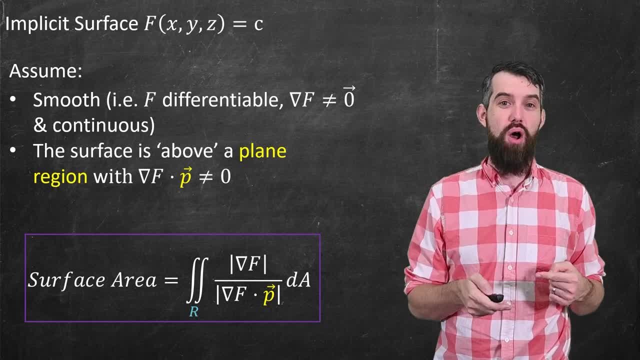 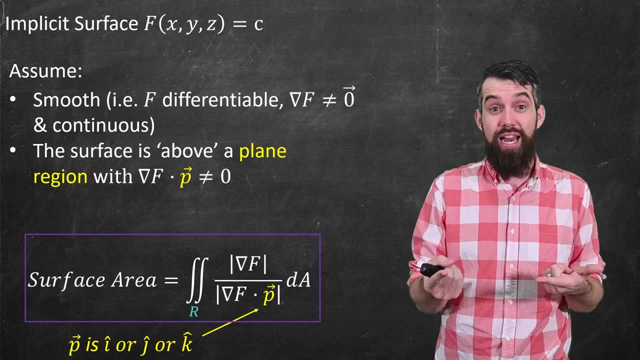 doesn't matter, And what I'm doing is replacing it with k-hat, with what I'll call a vector p-dot, and p here is just i-hat or j-hat or k-hat, As in, if you want to think of your region as a region over the y-z plane. 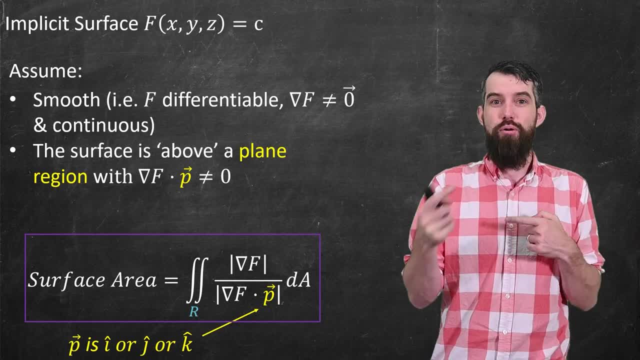 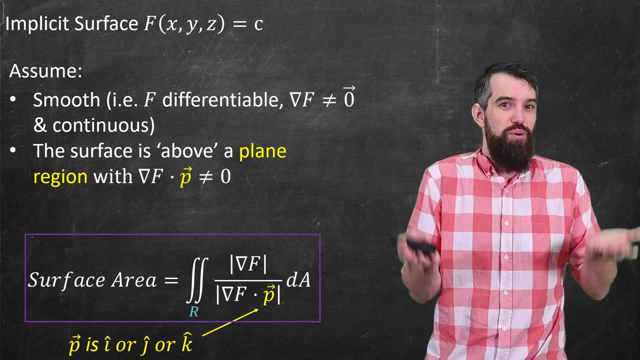 and dot it with i-hat. that's totally fine too. Or a region over the x-z plane and dot it with j-hat. that's also totally fine. For the most part, I just do it over the x-y plane with a k-hat. 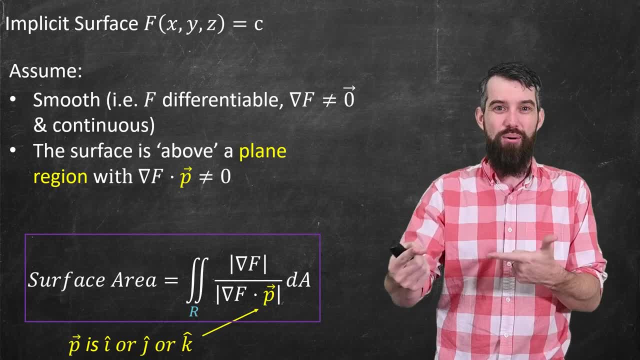 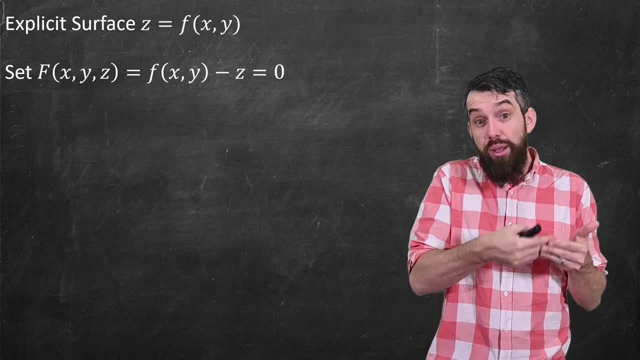 If it wasn't that, then you could just permute your symbols until it looking that way, if you wanted to. It doesn't really matter, But I just wanted to note that this statement can be said with a little bit more generality. So that was our formula for implicit surfaces. 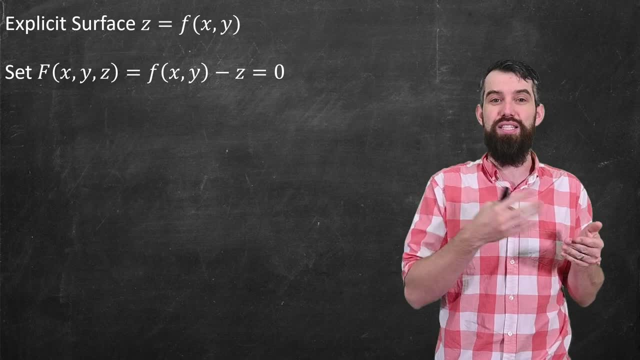 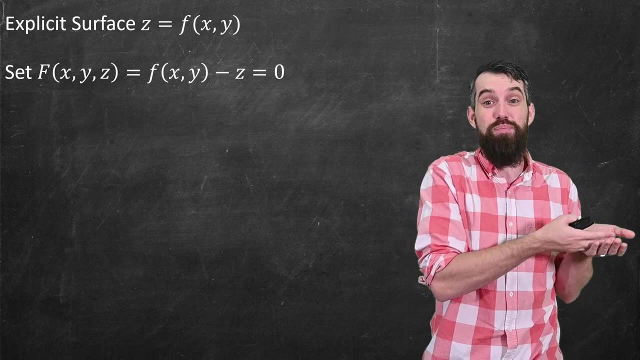 But now I want to do a formula for explicit surfaces. z is a function of x and y And really what we're going to do is just say every explicit surface can be thought of as an implicit surface. So, for example, I can come up with a capital F of x, y and z. 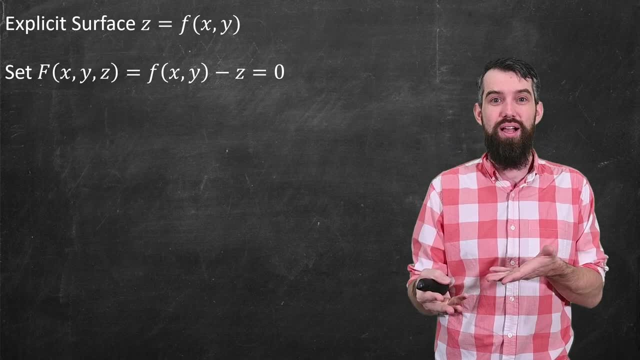 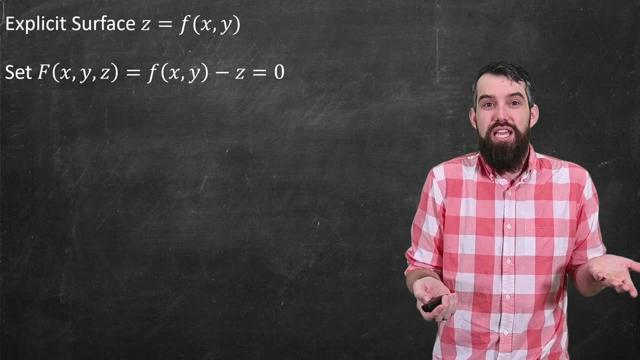 which is just f of x, y minus z, equal to zero. So the level surface to capital F is just the same thing as this explicit surface. Okay, And now I'm just going to plug it into the formula that I had. So what's the gradient of big F? 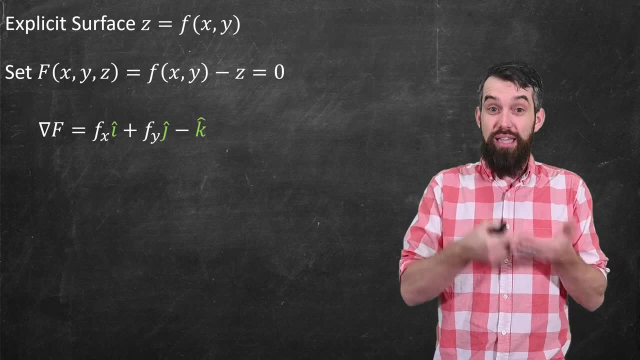 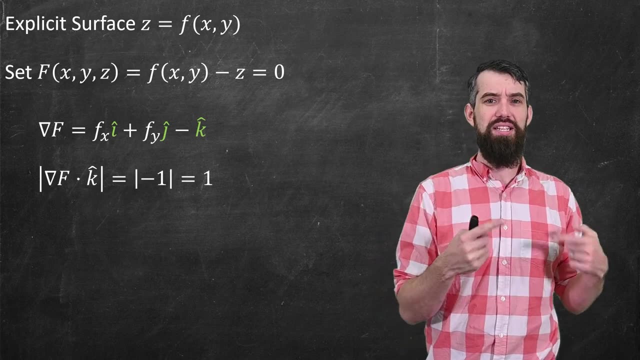 Well, it's partial of little f with respect to x in the i-hat, partial of little f with respect to y in the j-hat, and then minus z turns into a minus one in the k-hat. The length of f dotted with k-hat is pretty simple. 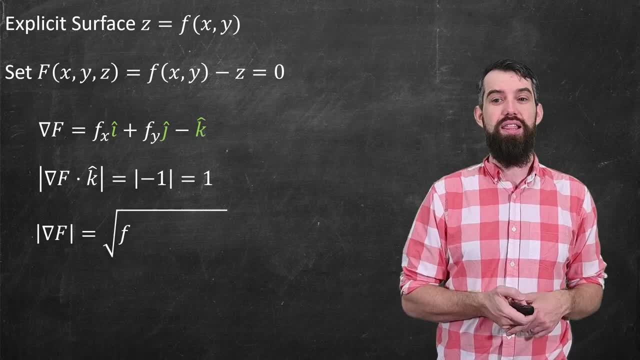 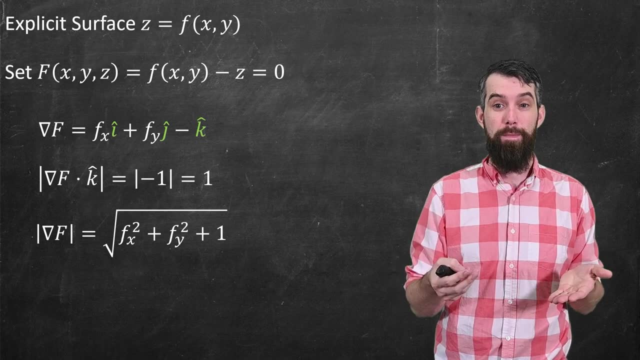 It's just like the minus one, which is one, And then the length of the gradient of f squared root of some of the components, So square root of fx squared plus fy squared plus one. So our formula that we just were talking about is the double integral over the region of this fraction. 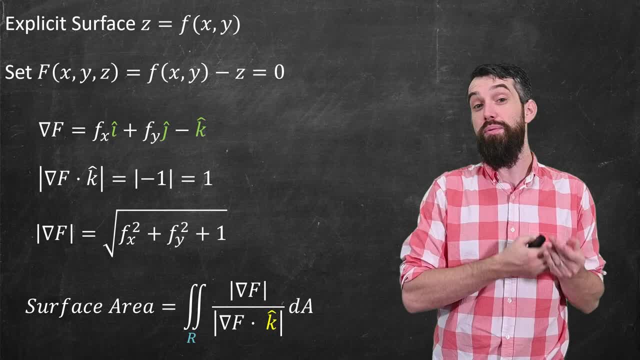 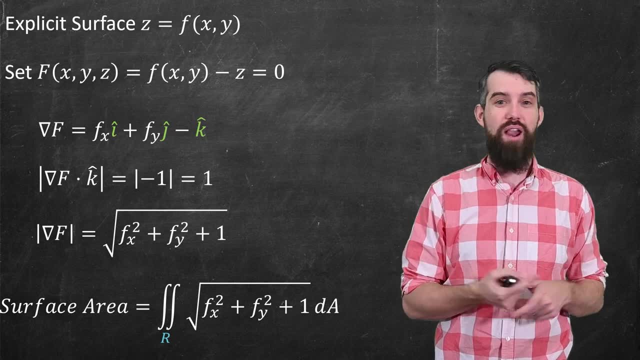 the length of gradient of f over the absolute value of gradient of f, dotted with k-hat, And so just plugging those two things in. well, on the top I get the square root of fx squared plus fy squared plus one, And on the bottom I just get one. 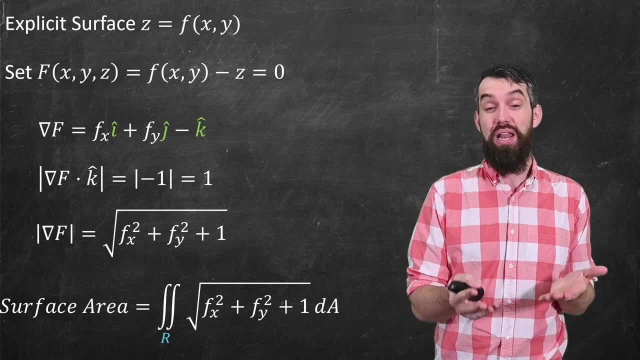 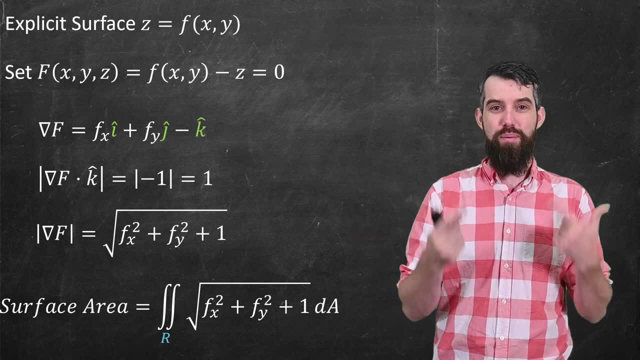 So I won't even bother writing it down. So this is our surface area formula for an explicitly described surface, And it's entirely up to you whether you want to have a new formula that you actually have to memorize every time, or if you only memorize the.